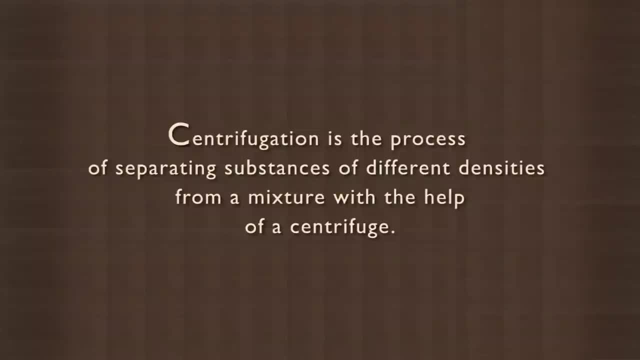 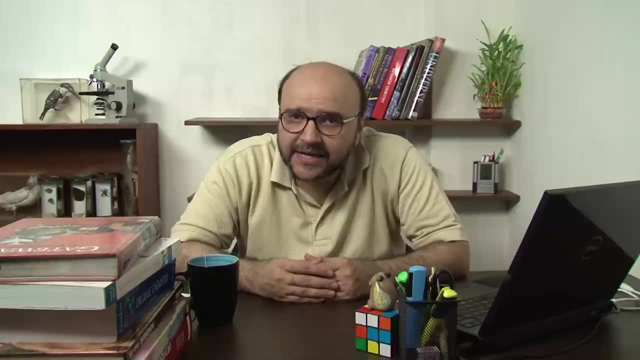 to quicken the process of sedimentation. Centrifugation is the process of separating substances of different densities from a mixture with the help of a centrifuge. Let us conduct an experiment to see centrifugation. For this we need a handy centrifuge machine. muddy water mixture. 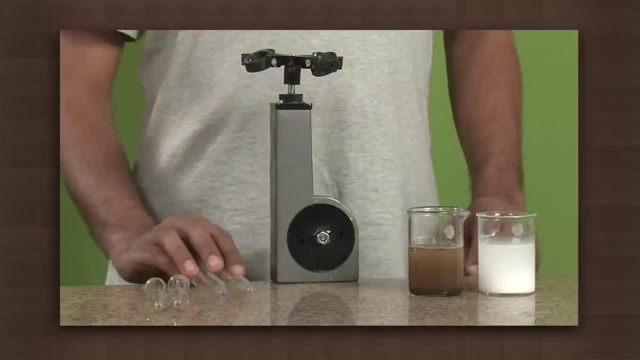 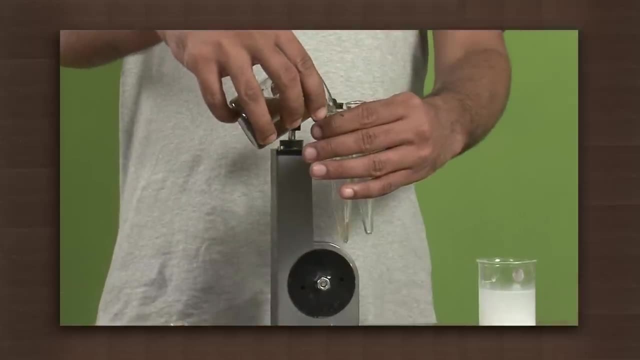 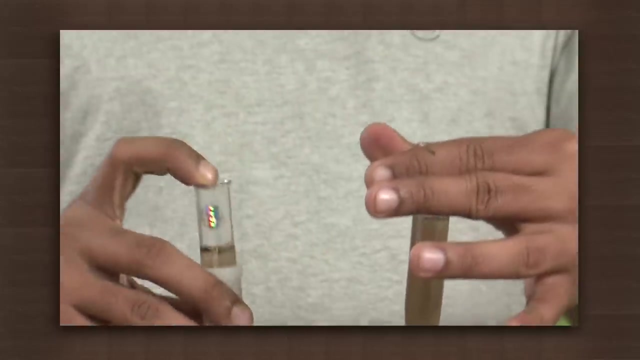 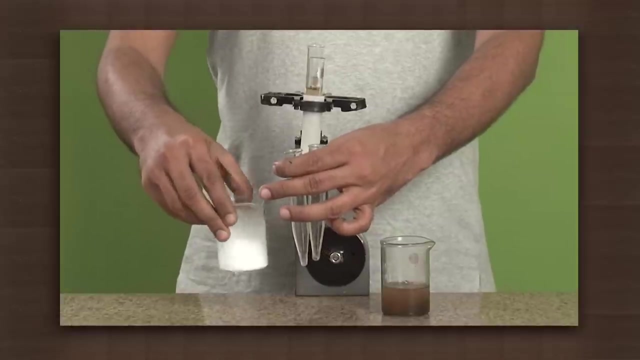 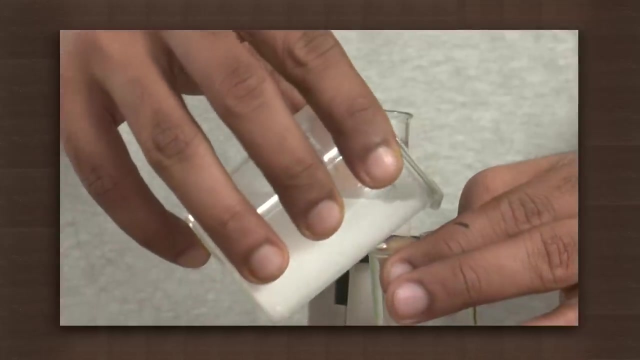 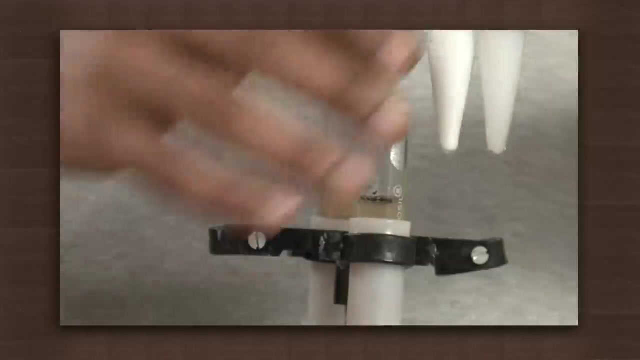 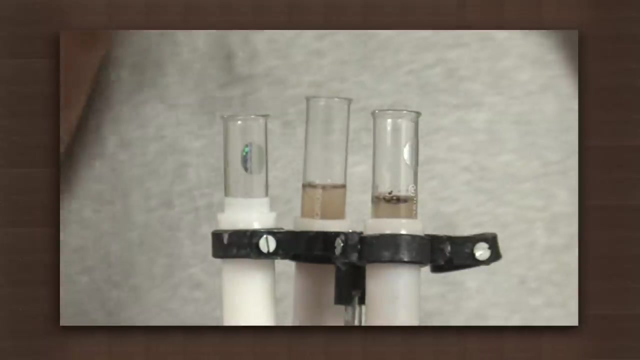 of calcium carbonate and water four centrifuge test tubes. Take the sample of muddy water and place the test tubes in the centrifuge machine. Now take the calcium hydroxide mixture in the test tubes and also place them in the centrifuge machine. Rotate the machines fast for few minutes. 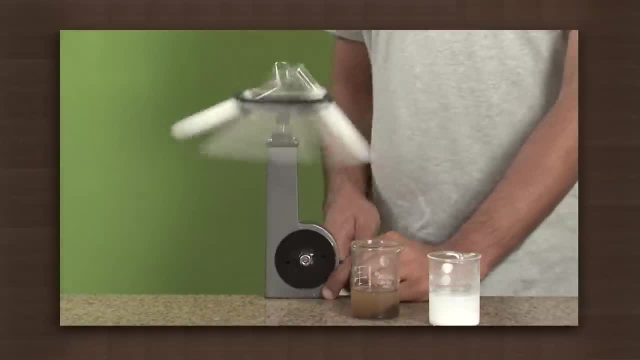 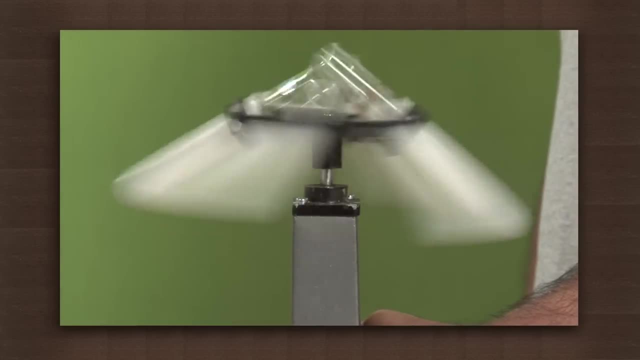 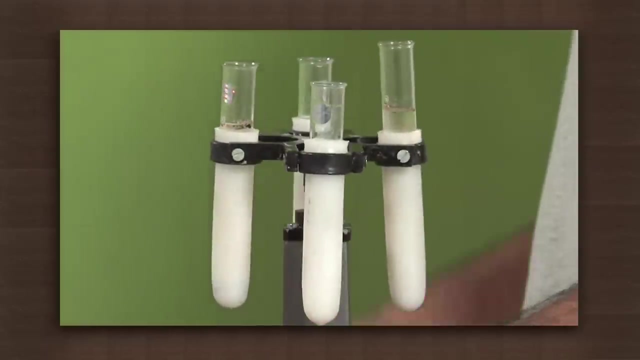 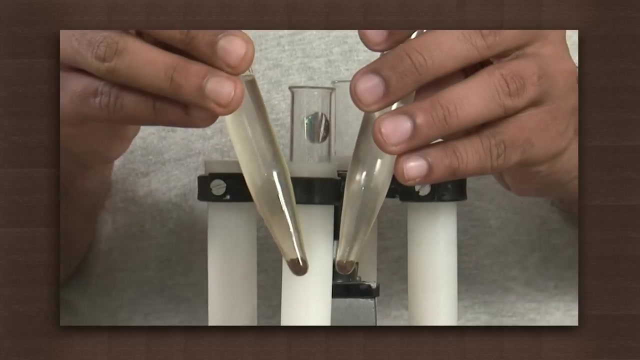 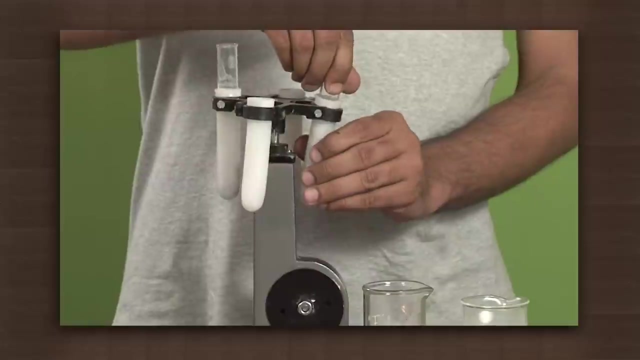 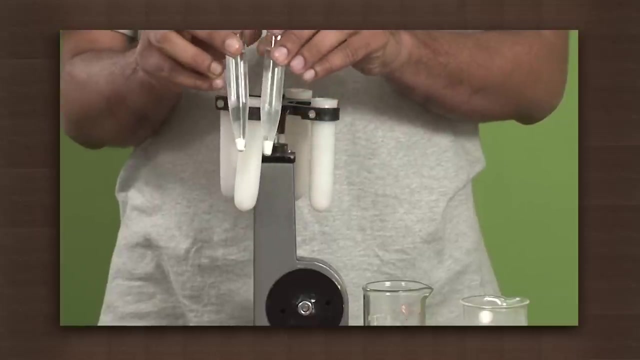 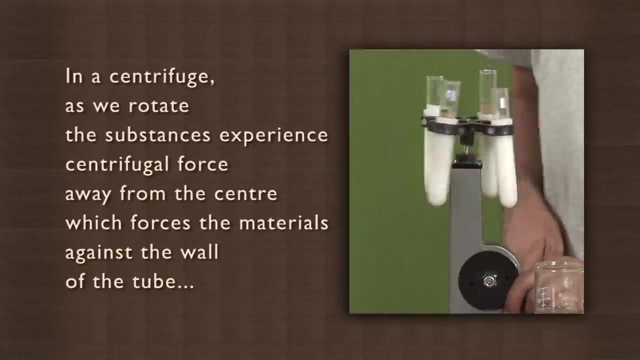 Stop rotating, Remove the test tubes and observe. We see mud particles and white precipitate have settled in each of the test tubes. This is the process of centrifugation In a centrifuge. as we rotate, the substances experience centrifugal force away from the centre, which forces the materials against. 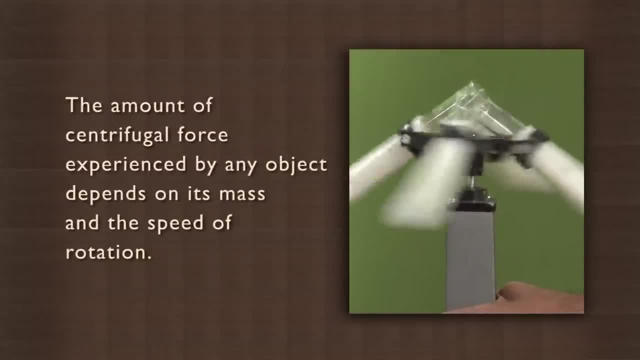 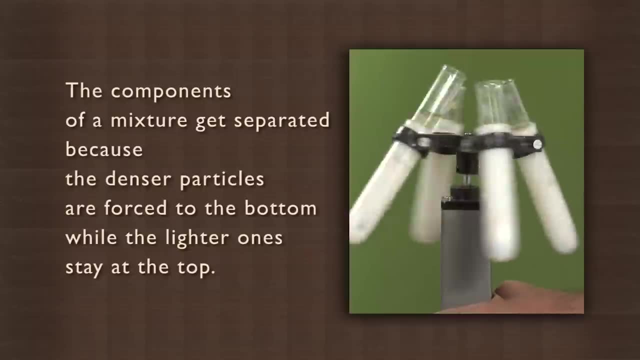 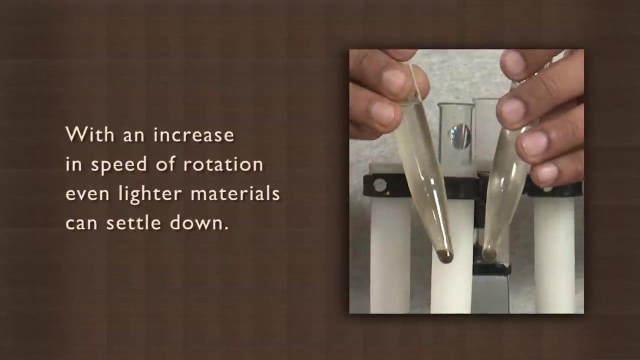 the wall of the tube. The amount of centrifugal force experienced by any object depends on its mass and the speed of rotation. The components of a mixture get separated because the denser particles are forced to the bottom while the lighter ones stay at the top. So with an increase in the speed, 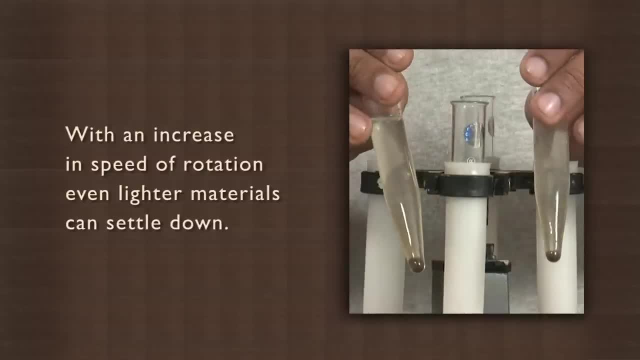 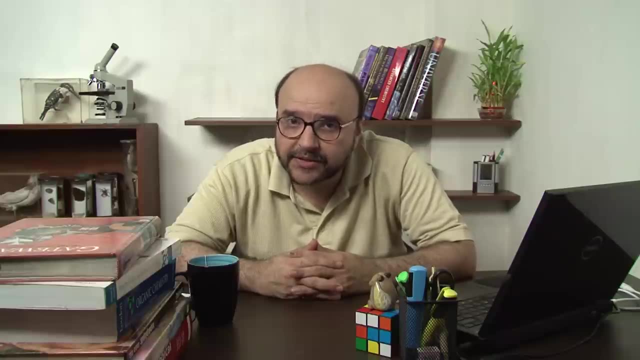 of rotation, even lighter materials can settle down. Centrifugation is used in diagnostic labs for blood and urine tests. It is used in dairies and homes to separate butter from cream.